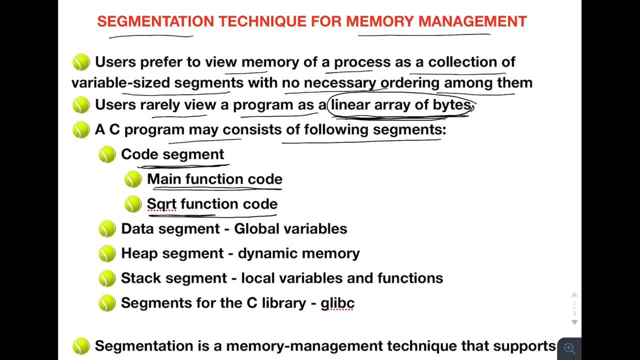 then you have a segment for square root function code- right. similarly, for other functions also, you can have different segment. then you have data segment- right. so this data segment stores all the global variables. both initialized as well as uninitialized global variables are stored in data segment. then you have heap segment- right. this. this has all the dynamic memory allocations, so 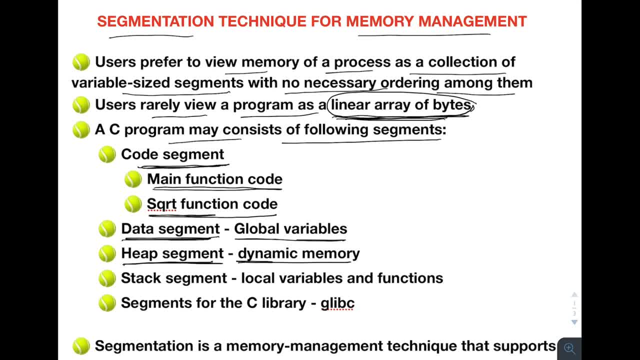 all the dynamic memory allocations are done in the heap segment. then you have a stack segment. so this stack segment store the local local variables as well as the function calls. all they are stored in the stack segment. and then also you have segments for the c library, right? so if it is a c, 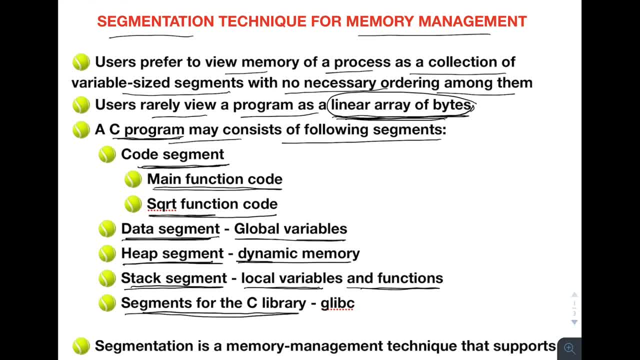 program: right, it will use a lot of library functions, right? so the library functions are actually a part of the c library that is called glibc. so in linux, this glibc- right, this is the. this is the c library. that hope that holds the code for all the library functions in c. 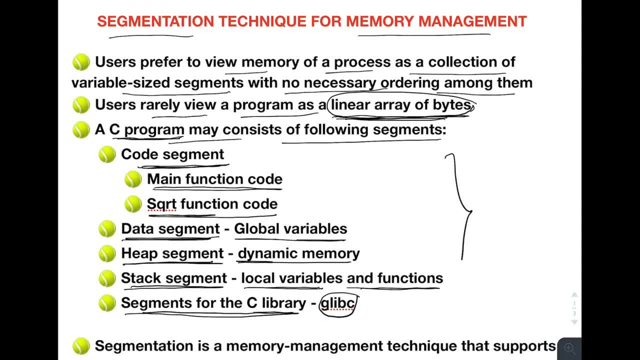 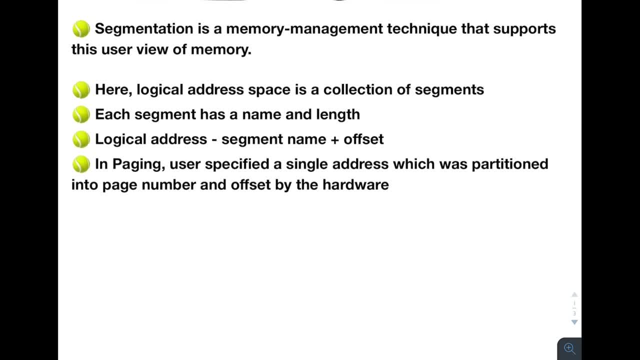 so these are the different sections which you will get when you write a c program and compile it and spell it in analyze code and apply a very simple method called 90. Expedition is a memory management technique. right segmentation has multiple segments. you start with logical address llama body, it takes DNA and memory董 go to theossen, the domain number glutineous. 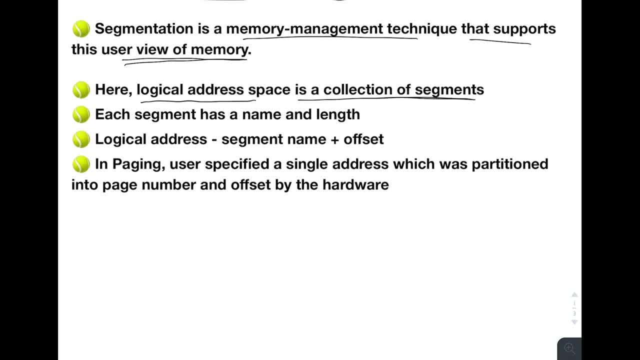 you operate only a dry database, not a unit. so this memory Taiashing can be created based on two different kinds of memory: Na ii, usually of memory override database. you copy one iPod, the other in the environmentnem ветirp of memory flip. Bastion for number of вкусm nest ik datum newspapers. 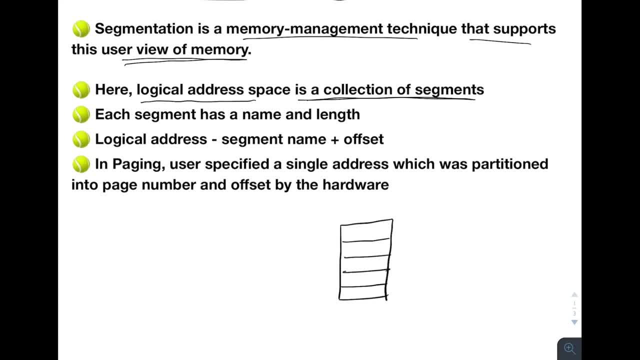 pages, right. But in this case, in the case of segmentation, the logical address is divided into multiple segments. right, There are many segments. this is segment 0, right. Here it was page 0, right. That's what the difference here is. Now, each segment has a name and 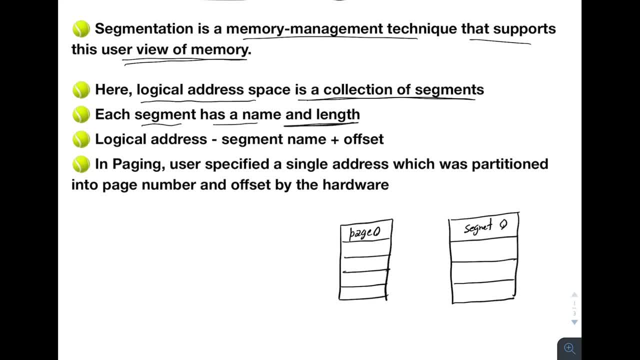 a length right. So in the paging concept each page only has a number right. So this is page 0,, this is page 1,, this is 0,, 2,, this is 3,, this is 4,. right, And there was I mean. 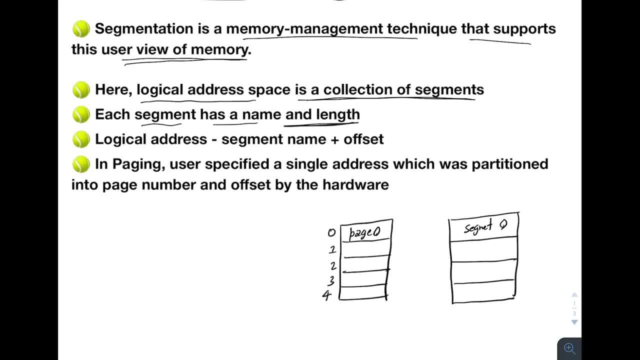 the length of this page was fixed by the kernel itself, right? So I mean in the paging concept, but it's different in the segmentation. So in the segmentation what happens? Every segment will have a name. So name can be number itself, right? So this is segment 0, this is segment. 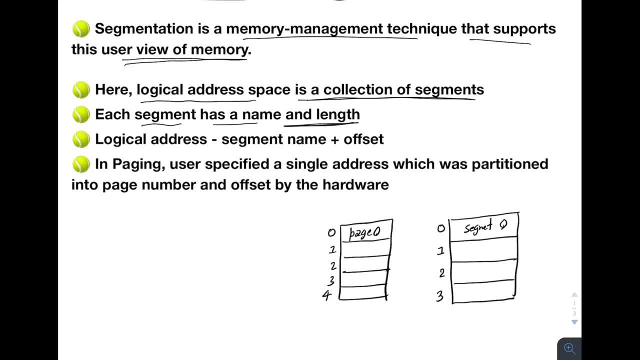 1,. this is segment 2,. this is segment 3.. And also every segment also will have a length associated with it, Because in paging every page was having the fixed length right, But in this case it's not the same Each. 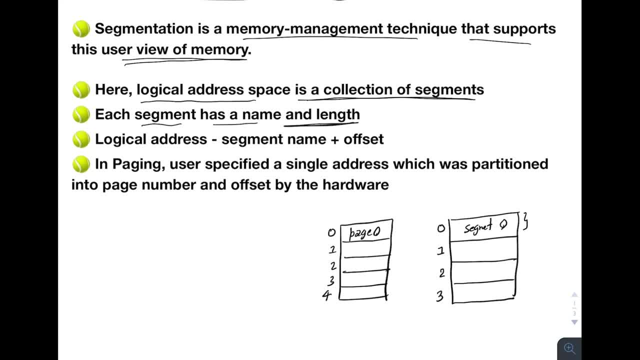 segment can have different length also, right. So you also need to define the length of each of this segment here. So basically, here you have, I will discuss it. So basically, logical address here has two components. One is a segment name, other is the offset, right? 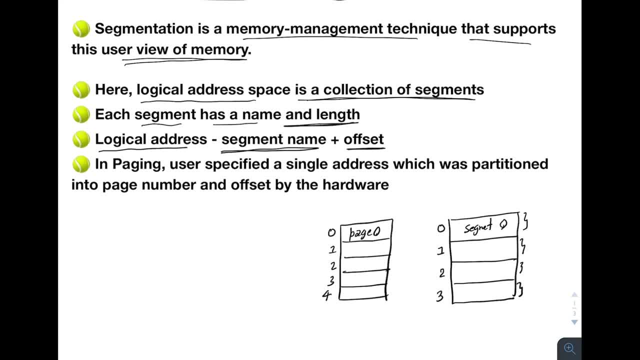 In the case of logical address- right I mean in paging. so in paging also there was two components: right Page number and offset right. But if you remember this page offset and the page number, it was the job of the Kernel. 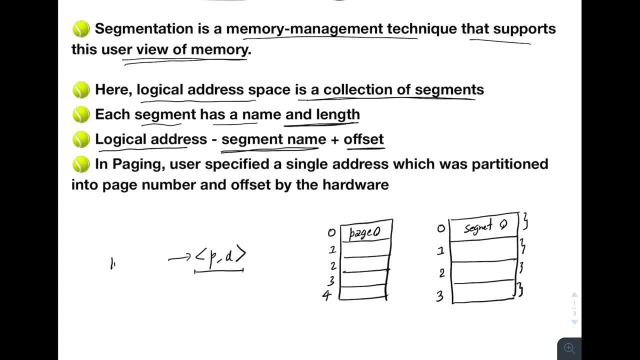 to decide this from the logical address. So the programme only provided the logical address, And from the logical address the Kernel has to decide the page number and the offset. But in the segment um segmentation kit that's not the case. In the case of segmentation the process itself has to provide both the segment. 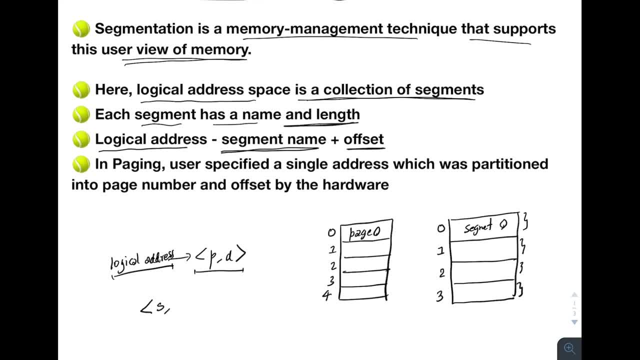 as well as the offset, Both it has to provide. So both of these components has to be provided by the process itself. In case of paging, the process only provided the logical address and then kernel broke down the logical address into two components. So this is very important. 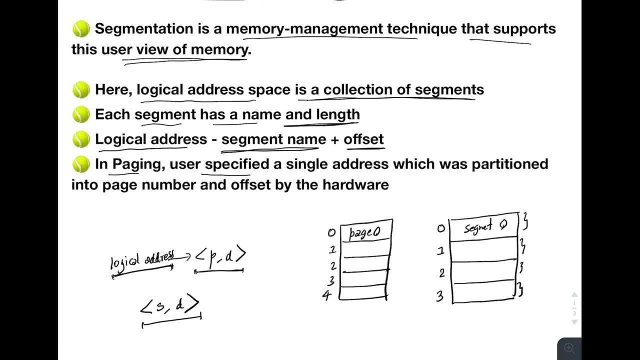 to remember. So in paging user has specified a single address which was partitioned into page number and offset by the hardware. So in paging this was done by the hardware. But in segmentation this has to be done by the user process itself. So user process has. 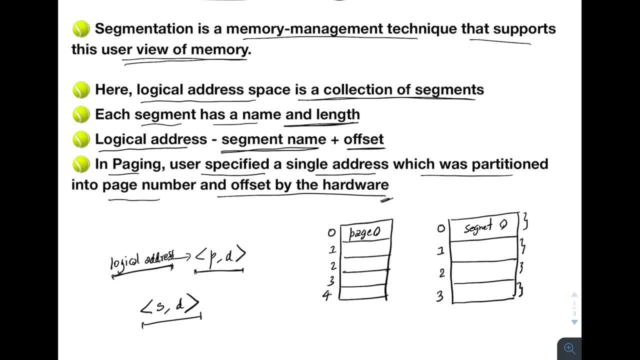 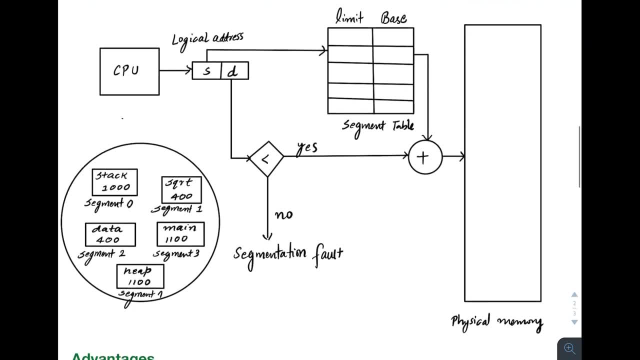 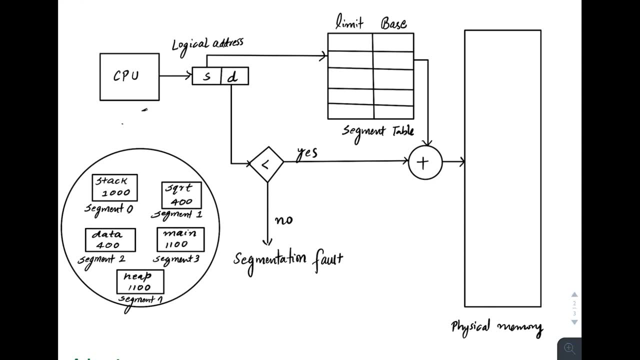 to provide both the segmentation number as well as offset for each segment. Now let's go and understand segmentation with an example. So here also you have the CPU, right, I mean to the CPU. So here you have the CPU. So here you have the CPU. So here, 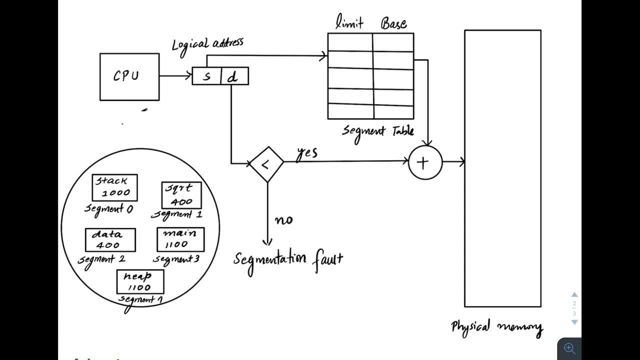 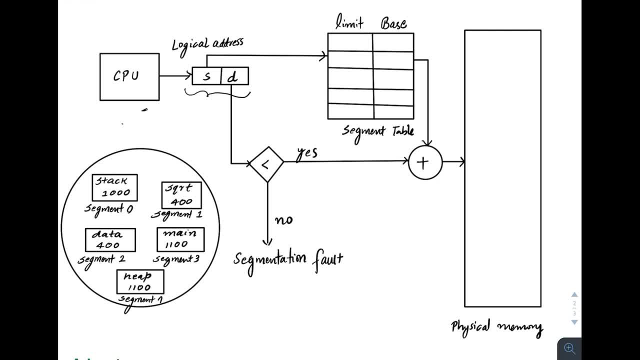 segmentation number as well as the offset right. Both will be provided by the process itself Now. so, if you remember right, in case of paging, only program counter was there, right, Program counter was there, and now CPU. what CPU used to do is CPU used to start. 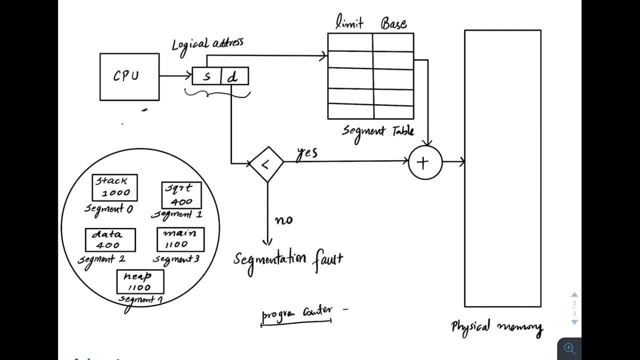 executing from this program counter right, And this was a logical address. So it can. So the process only provided the program counter. that was as a logical address. But in case of segmentation the process has to store both of these components. I mean. 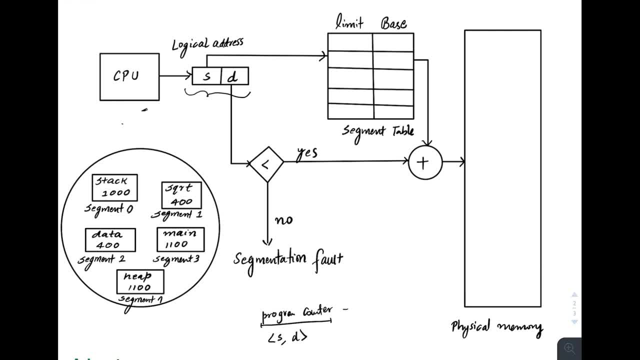 segmentation number as well as offset, and it has to provide this for execution of the process. Now, this is the segmentation number, D is the offset, right, And now similarly. so what will happen is: first we need to, so Cuddle also needs to. 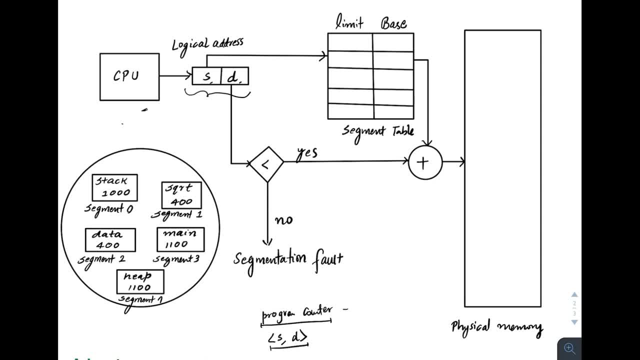 provide the memory protection, right? So basically what we are doing here is we are checking this offset, right? So what is offset here, right? So basically I will just explain that also. So basically, let's say: this is the stack segment, right? 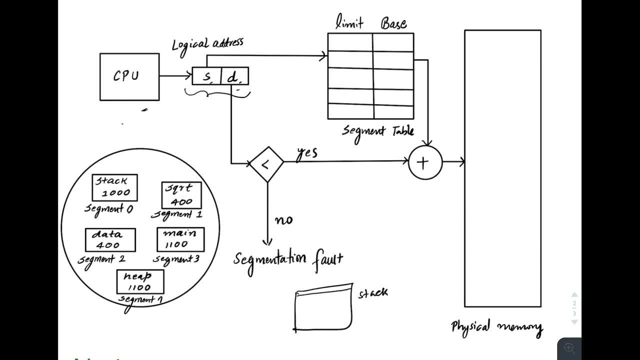 This is the stack segment. Now, this will have many bytes right, So I am assuming that the memory is byte addressable. it will be broken down into multiple bytes right. Zero. this is one. two. this is three. 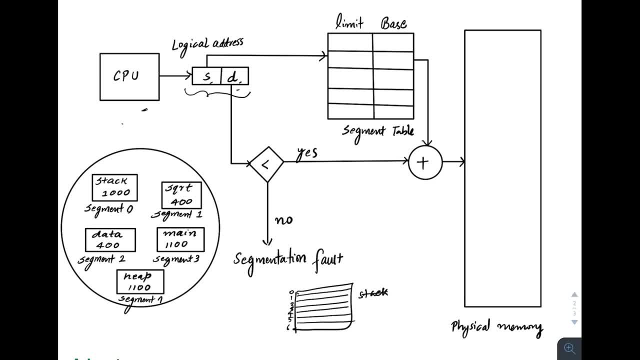 Now, initially, let's say okay, let's say this is the okay main, this is the main segment. let's say main function segment right, Actually, execution will start from the zeroth byte right. And for the main function, let's say the segment number is three. 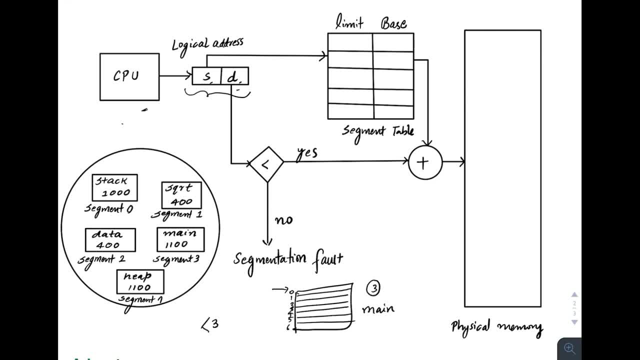 So initially, basically, process will provide three and initially the offset will be zero, right, Because in the main function initially it will start with zero offset, right Once this offset, I mean the instruction at this offset, is executed by CPU. next it: 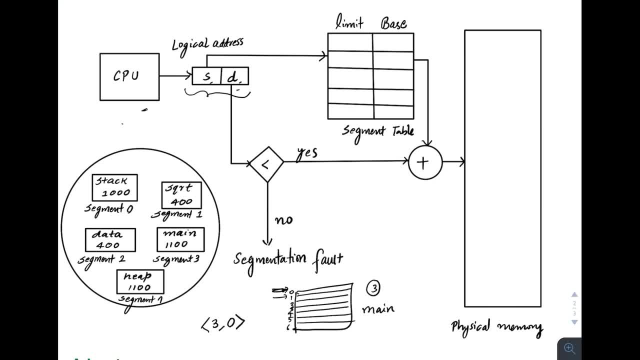 will move to the first byte right. So now this will change from zero to one right. Similarly, it will go to two, three, four, five, six right. So these are the offset values. right- Offset means the displacement within this segment, right. 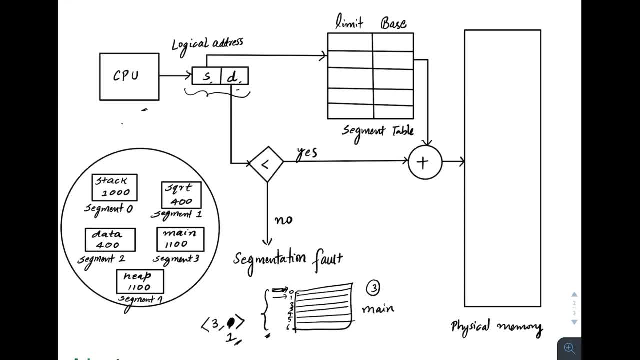 Initially. but initially the displacement was zero, then the displacement of one, then it will keep on increasing right. So this is the offset Now. first you have to check right for memory protection that this offset right it is. 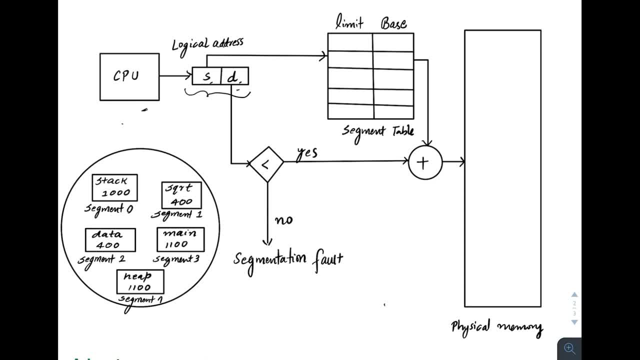 actually lesser than the okay. first we have to explain the segment table, then I will, then I will explain the memory protection right. So okay. So in in case of paging right, there was page table, right. 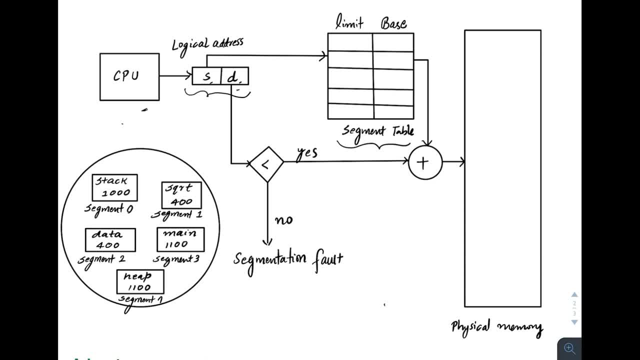 So in terms of, I mean in case of segmentation, we have segment table. So basically, what we have here is, for every of the page right, we have a limit register. I mean the value of, I mean segment limit and segment base. 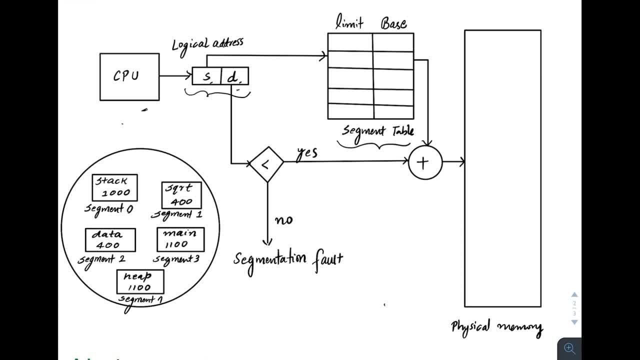 So I'll explain what are these. So limit is nothing, limit is the size of that segment, right? So I have taken an example here. I will fill in the values here. So here we have five segments, if you see: stack segment, square root segment, data segment, main segment. 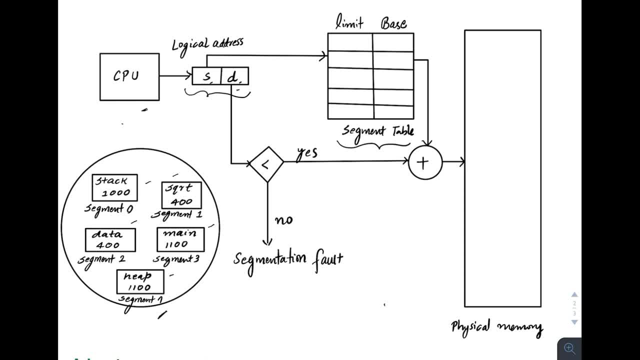 and heap segment And inside this this value is the. I mean this. 1000 is the size of this stack, 400 is the size of the square root. Similarly for others also. I've written inside the box the size of those segments and also. 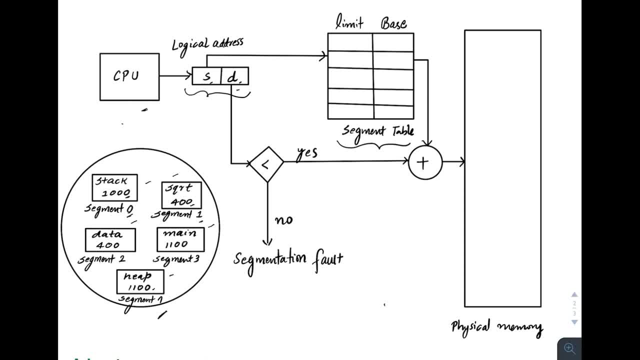 I've given number to them. segment zero is stack. segment one is square root, right. So basically this segment table for each segment. so zero one, two, three, four. So in paging, if you remember, these were the page numbers, right. 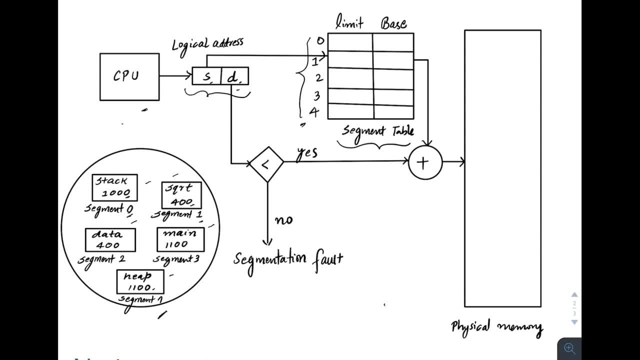 But in case of segmentation, these all are the segment numbers And limit is basically the size of each of these segments. So what is the size of segment zero, that is, stack, that is 1000,. segment one, it's 400,. 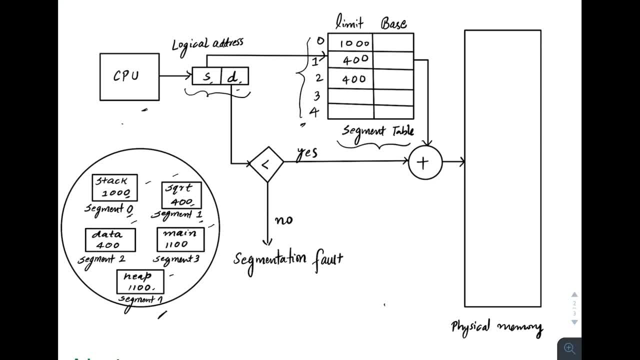 segment two: again 400.. So these are 400 bytes. okay, 1100.. This is also 1100, right. So we got the- I mean the limit values for this, right. So segment limit basically contains the size of that segment. 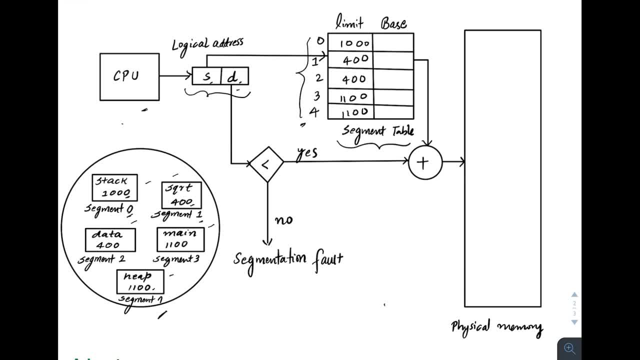 Now, what is this segment base? So segment base is the. so now, basically, the kernel will decide to put this, I mean segments, into the main memory, right? So basically, base, segment base is the starting address of this. 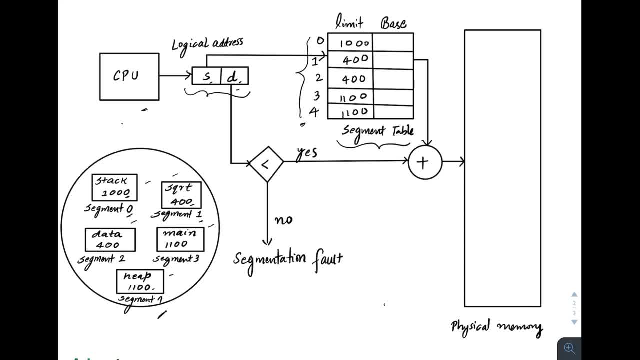 Segment in the physical memory. So I will just explain this with you an example. So let's say the base of this was, let's say, 1400.. So the kernel will decide this. So the kernel will basically allocate this, I mean this segment, into the main memory. 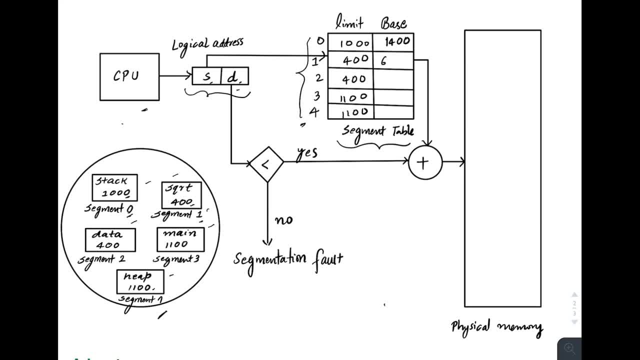 So it will decide by the kernel itself. what is the base address? 6300, 4300.. This is 3200.. And this is, let's say, 4700, right, Let's say these are the base address that the kernel has filled, right. 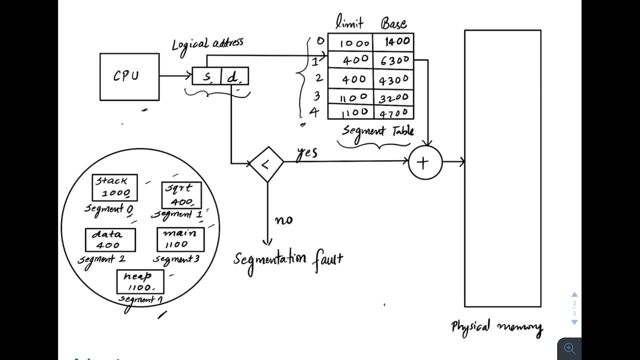 So this actually means that the segment 0 will start from 1400 in the main memory And this is segment 0.. So basically, base address means the starting address of this segment In the main memory, that is, 1400.. 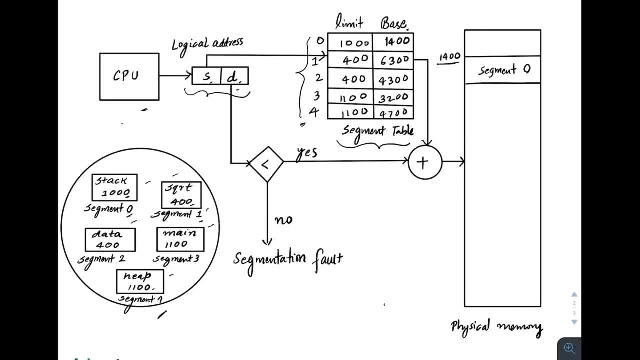 And this will be decided by the kernel. And what is the size of this? Size is 1000, right. So it will go from 1000 to 2400, right? Similarly for, let's say, segment 1, it is 6300, right. 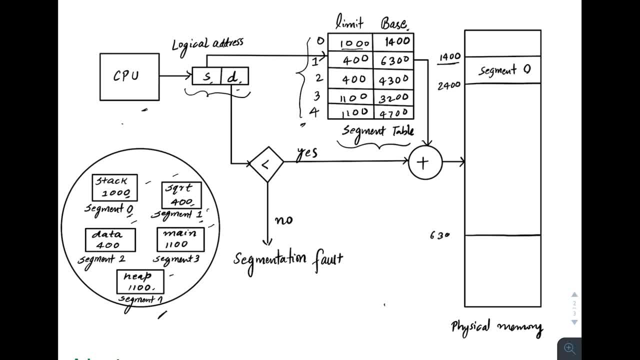 So let's say, here it is the address, 6300.. And segment 1, this will go from. and what is the size of this? It's 400.. So it will go through 6700, right. Similarly for others also, you can fill. I will fill for this second also. 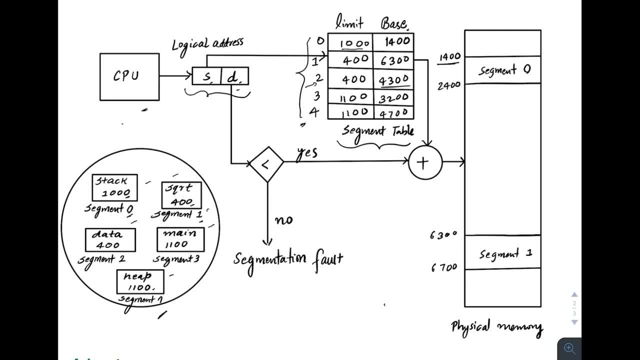 The starting address in the physical memory is 4300.. Let's say it's here 4300. And it will go till the size of this project: 400, 4700.. Like this is segment 2.. Similarly you can fill the I mean for the other two segments. 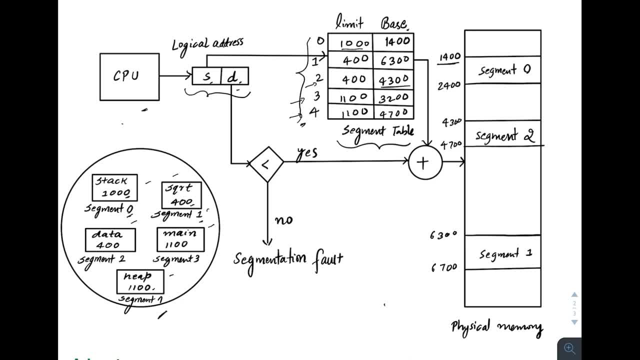 Also, you can allocate the memory in the physical memory right. So this base segment base address is provided by the kernel, Because kernel knows that which of the physical memory are free right, Which areas of physical memory are free. Depending on that, it will provide a starting address for each of the segment. 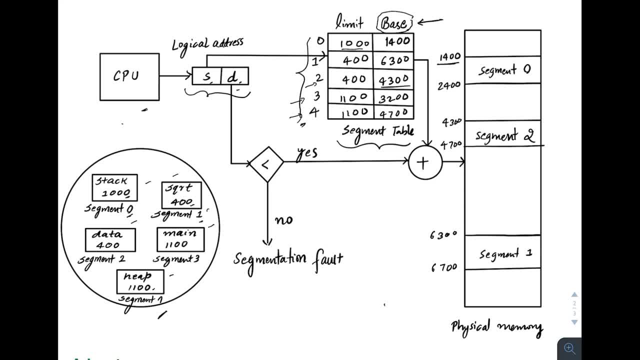 Now I was talking about the memory protection, right? So I will go to the memory protection again now. So, basically, if you know that, right? So we know that, what is the size of the process by using this limit segment, limit value in this segment table, right? 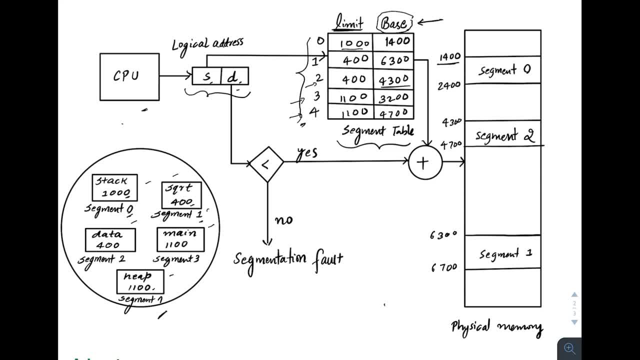 So let's say, if a process is trying to access some memory outside this, So see this. So this is just segment 0, right, And it can start from any address. right, Let's say, in the logical view, it will start from 0. 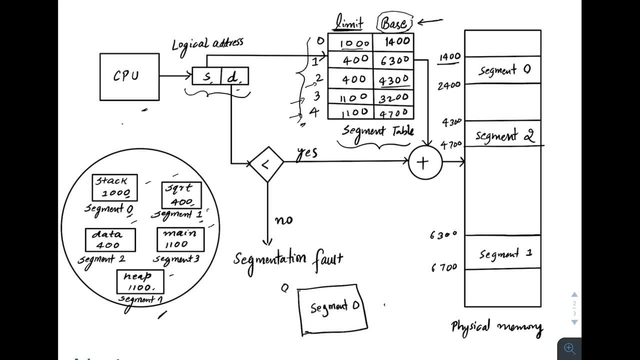 I am talking about logical, Not the physical view. In the physical address it is starting from 1400., But according to the user it will be starting from 0.. And the size of this is 1000.. So this will go till 1000, right? 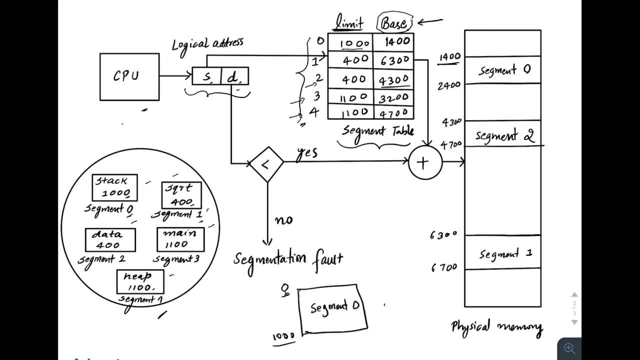 So it will I mean 0 to 999,. actually it will be right, Because we are taking base as 0.. So it will be 0 to 999, right? That is 1000 bytes, right. 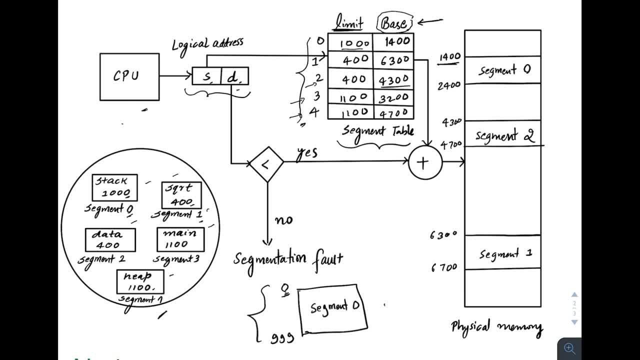 Total of 1000 bytes. Now, let's say, if somebody is trying to access the 1000 bytes, right. 1000 bytes, right. This segment 0 is trying to access the 1000 bytes, But this 1000 bytes does not belong to this process, right? 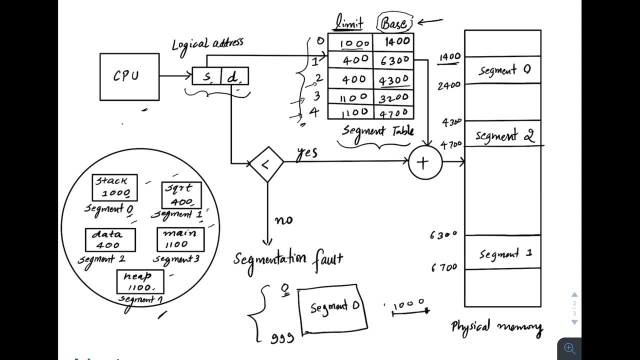 Because this process only extends from 0 to 999,. right, And this 1000 bytes will be for some other process, right? That does not belong to this process. So in that case, I mean the CPU will inform the kernel about the. I mean that it is trying to access some other memory that does not belong to this process. 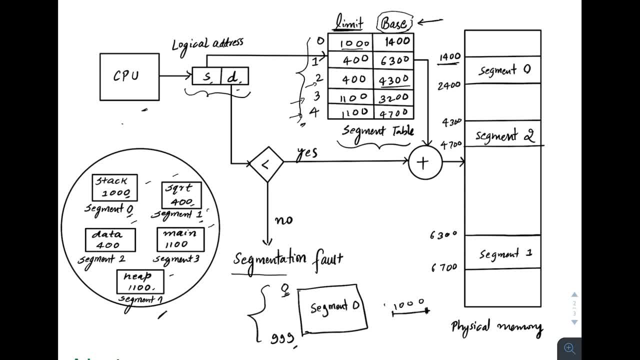 And then the kernel will basically send a signal to this regarding the segmentation fault. So that's what we are checking here, right? So if this d is smaller than right, So if it is smaller than the limit, right? So if you see, this 1000, right is not smaller than this limit value of 1000, right? 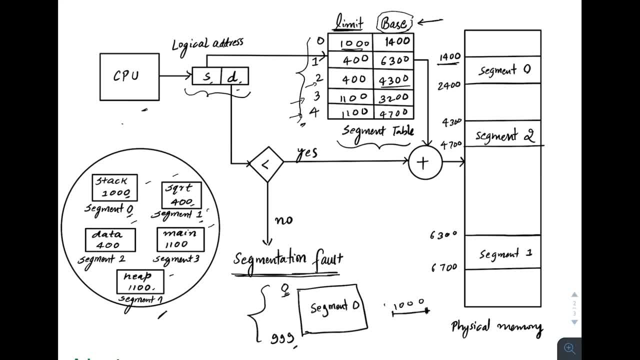 It is equal, right. So in that case segmentation fault will be raised by the kernel. But if it is smaller, let's say the value here was displacement 0, right. So the value here was displacement. value was, let's say, some 500, right. 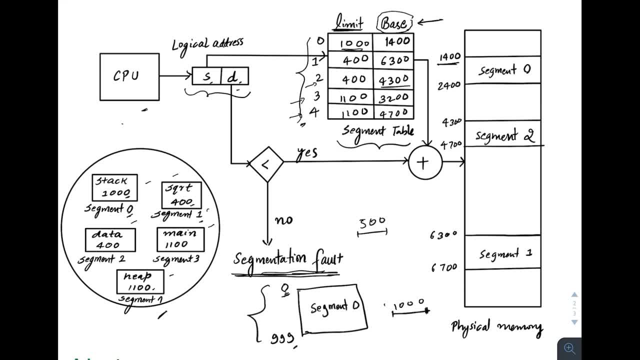 So in this case, 500 is smaller than 1000.. In that case now you have to map this logical address: 500, right Plus the segment number. that is 0, not 0,. yeah, it is 0.. 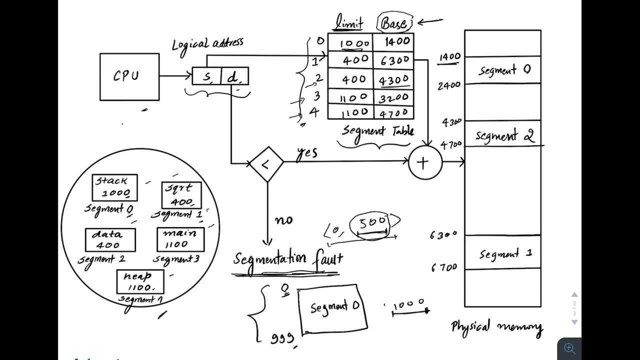 You have to map this to the physical address. So let's see how this mapping is done. So we have already talked about the memory protection. Now we will discuss about the memory mapping. Now, from here, we are getting the displacement. Sorry, we are getting a displacement from here, or the offset. 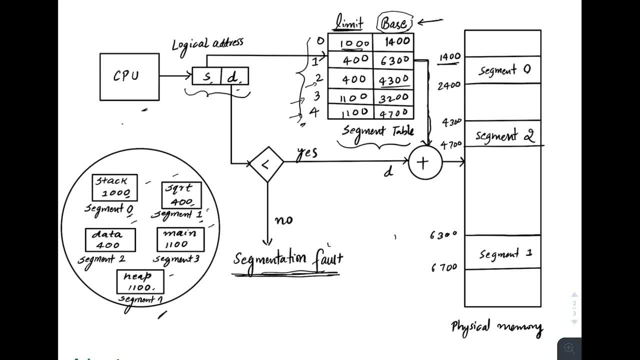 And from here we are getting the base, I mean the starting address of this segment, right? So if you basically add these two, if you add the offset with the base address of this segment, then we will get the exact physical address, right. 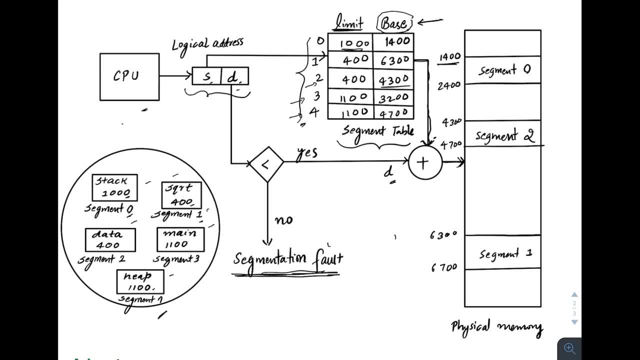 So that's what we were doing in other tech paging, I mean other memory mapping and other memory management techniques also, right? So basically, if you remember, we used to add the base address to the offset right In the paging. if you remember, each page entry, for each page, right a frame was allocated, right? 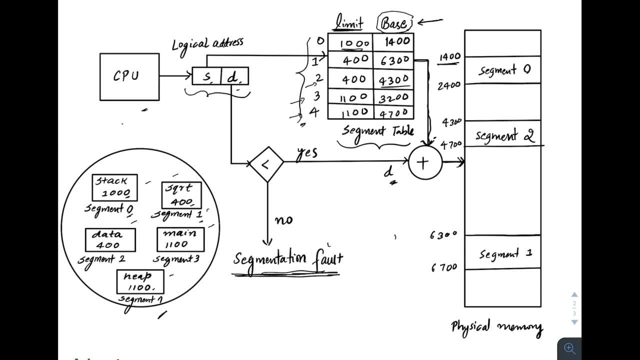 So we used to add the base address of that frame to the offset to arrive at the physical memory address. Similar thing we are doing here also. So that is the example here, what I have given here, And I hope you would have understood how segmentation works. 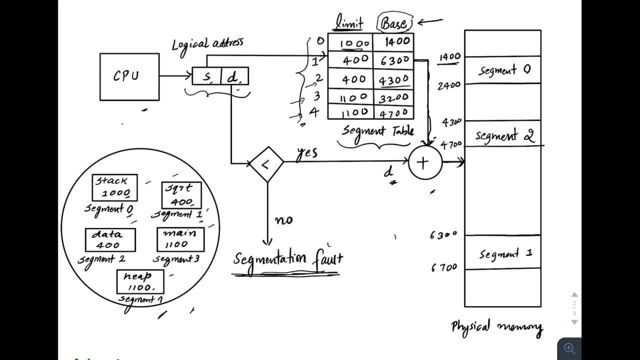 So this works same as the paging. So there are some differences here. So difference here is that I mean in the paging you have only the logical address And it was divided into P and D by the kernel. Here, process itself will provide the segmentation and the displacement right. 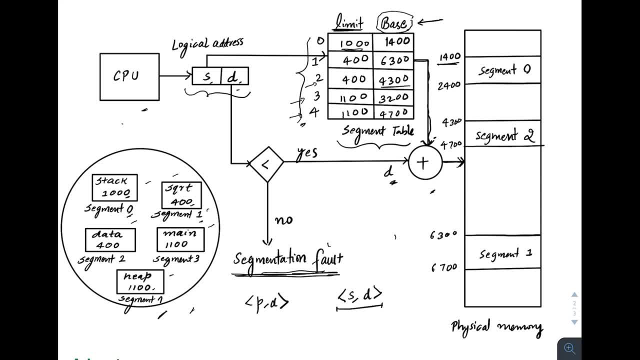 And in the paging memory protection was provided with the help of valid and invalid bits. right Here memory protection is provided Just by using the limit register, Not the limit register, the limit and segment limit values right that are already defined. 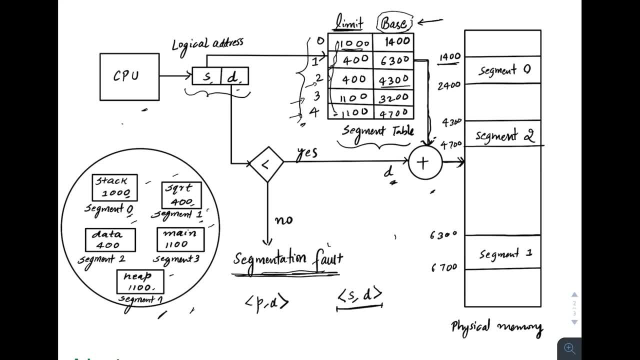 This is the length of the process. That's how memory protection is provided And how memory mapping is provided. It is provided by: so the kernel will fill the segment table with the starting address of each of the segment. You will add this starting address with the offset to arrive at the physical address. 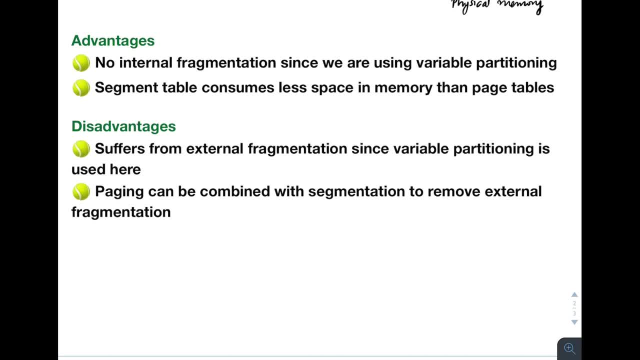 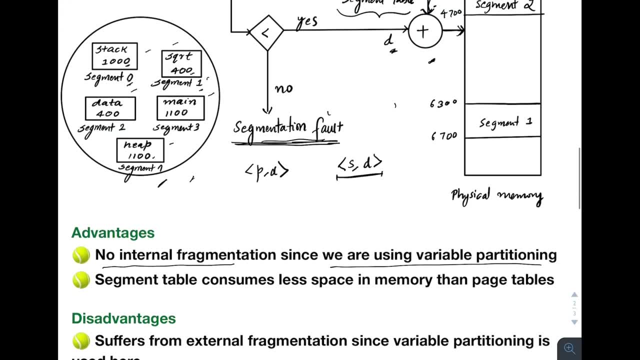 Now let's look at advantages and disadvantages. So the advantage here is that there are no internal fragmentation, since we are using the variable partitioning. So if you see here clearly right what the technique which we are using for memory partition is variable, right. 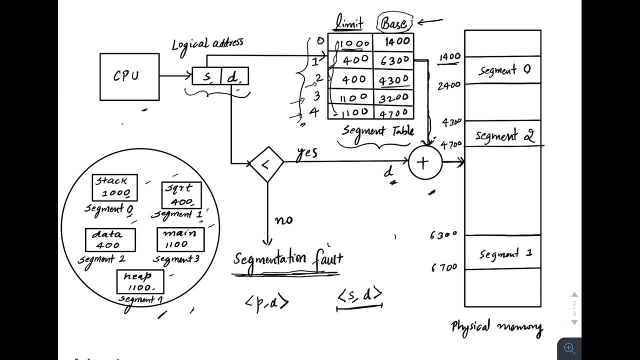 Since initially, I mean the whole of this RAM right was empty right, It was a whole, a complete whole right. Then we started dividing this whole into multiple chunks right And new holes were created right. So here, if you see, initially there was one whole. 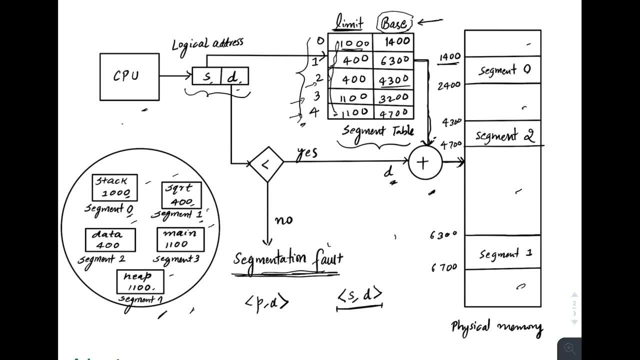 Now you have one, two, three, four holes right After this partition has taken place, right? So this is the similar concept of variable partitioning that we have discussed for the contiguous memory allocation. So the difference here is that here the process is broken down into segments, right. 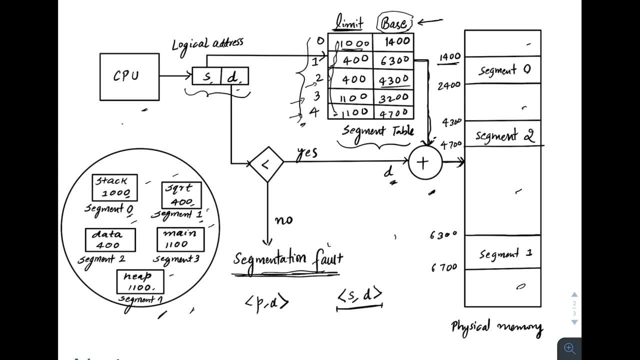 In the case of- I mean, when we are talking about the contiguous memory allocation, the process was not broken down into, I mean, this segment, It was a, I mean it was a complete process, right? So we need to fit that complete process into the physical memory. 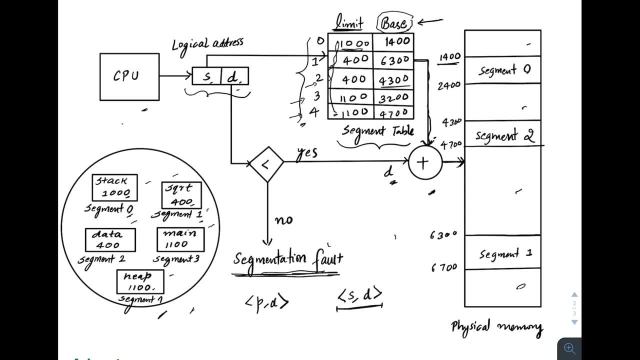 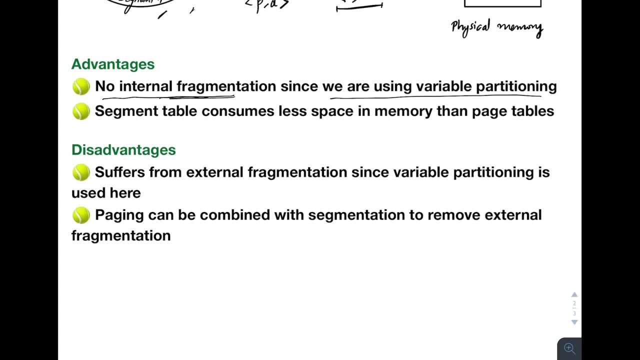 Here the difference is we need to fit the segments into the main memory. And the advantage. another advantage is- and also we already know that right- no internal fragmentation will be caused in the case of variable partitioning. right And advantage here is that segment table consumes less space in memory than the page tables. right. 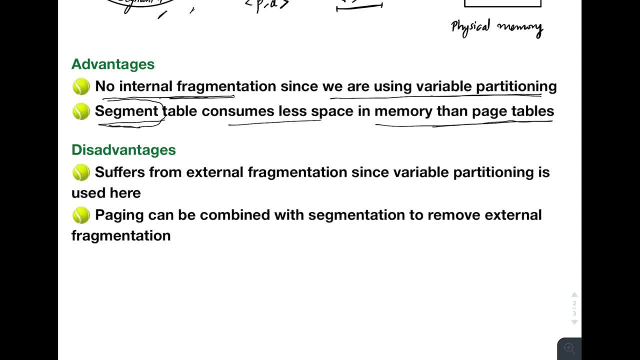 Because segment number of segments will be limited. right, You cannot have like a million segments. Right For a program. But in the page table entries you can have a million entries. right, Because you can keep on dividing. I mean, if you have a very large process then its logical address will be divided into a huge number of pages. 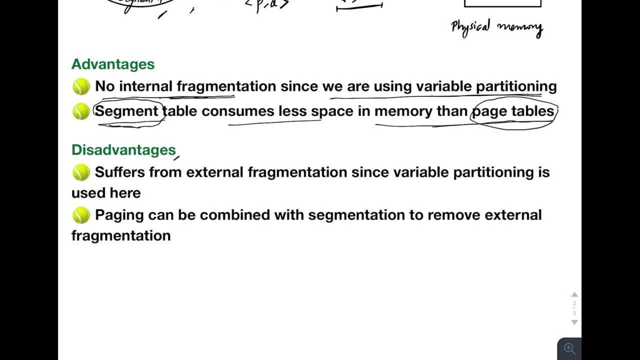 So what are the disadvantages here? So the disadvantage here is: so, if now you know that, right, It is using the variable partitioning, right? So basically, it will suffer from the external fragmentation problem, right, Since we are using the variable partitioning method.